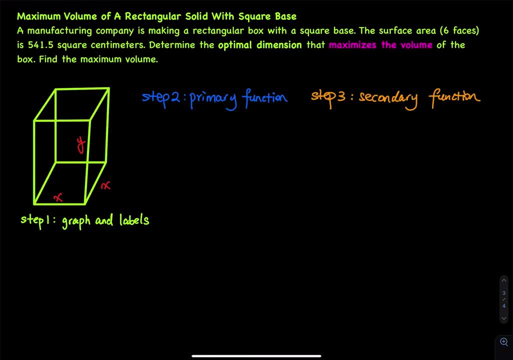 Rectangular solid, square base, and then the base is x by x and then the height is equal to y. Okay, so what's the primary? The primary function is: we are trying to maximize the volume. So what is the volume of this rectangular solid? So the volume is the area of the base times the height. 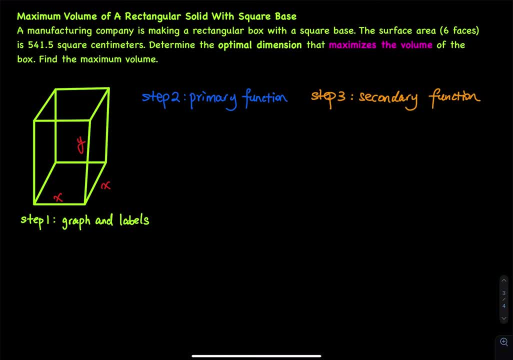 right. So the concept is: you find the area of the base which is x times x, so that is one square, And then you multiply by y. That means you are stacking up the square. So you have one piece of paper on your table and then you have to stack. 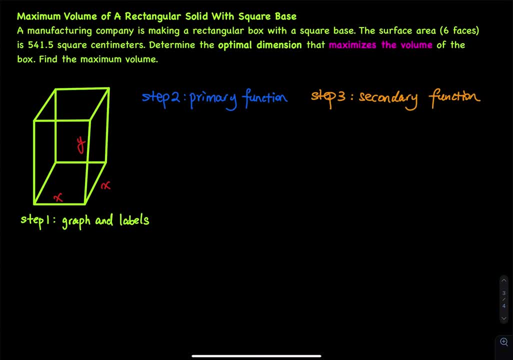 up this square. So how many copies of squares do you have? The answer is y copies. So when you stack them up that you have a 3D volume. So the volume is equal to you. so the volume is between x times. 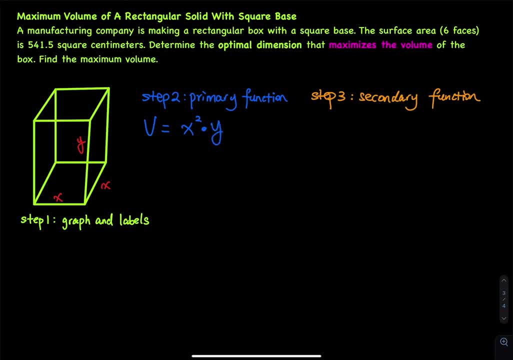 x and then the height is equal to y, And then I only call this a V. I cannot call this a V of x. this function has two variables, x and y. i cannot just take the derivative like that. that's why i have to figure out a secondary function. the secondary function is the given condition. 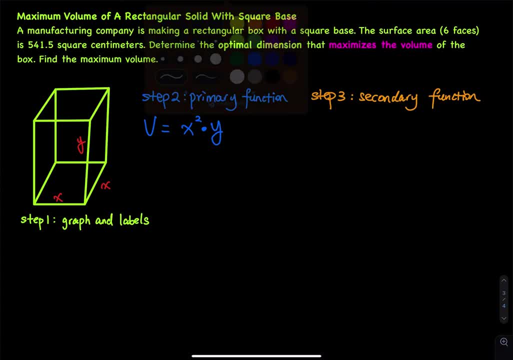 surface area. so how do you find the surface area, the surface area, i call that sa, so that is equal to. you have the top and bottom plus four sides right, so the top and bottom is x square. right, so x square. this is the top or the bottom. so you have a top and bottom. then you have to multiply. 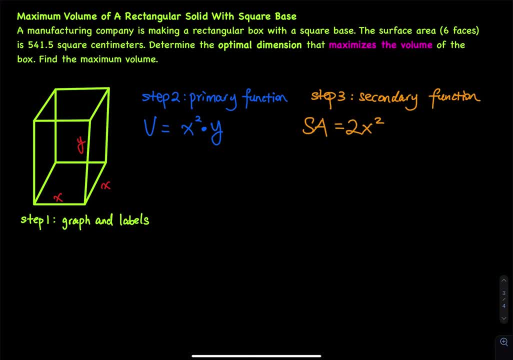 by two. x square is just one square. you have two top and bottom right, so you multiply by two. and then how about the side? i think they call that the lateral area, the side, the four sides. so the four sides, one right here and then one right here, one on the back and then one on the 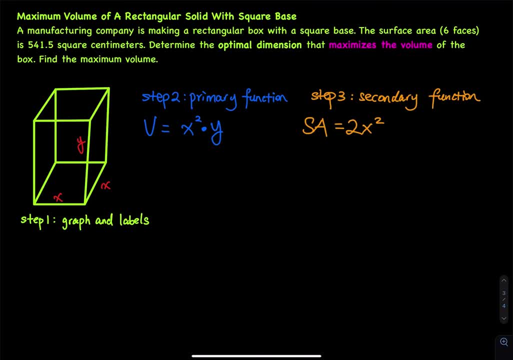 left the four sides. so the side is x by y right, and then you have to plus x times y. this is four sides. this is one side, and then you have four of this and then you multiply by four and then the surface area is 541.5, so 541.5 equals to 2x squared plus 4xy. let's isolate. 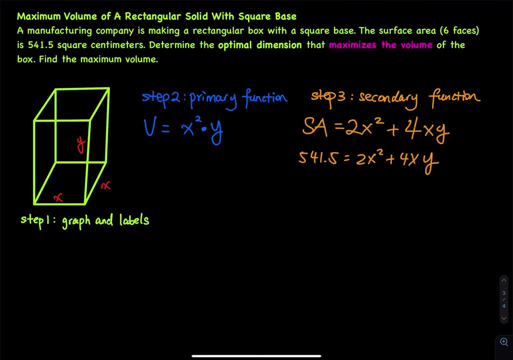 y on one side. so first we take 541.5 minus 2x squared, that is equals to 4xy, and then we divide both sides by 4x, so we have 541.5 minus 2x squared divided by 4x, that is equals to y, and then I. 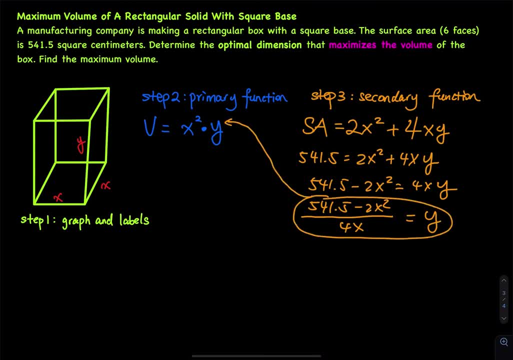 will plug in this y over here and then I can rewrite the primary function, that is: equals to v of x, equals to x squared times the y, which is 541.5 minus 2x squared divided by 4x. and then let's just use a big parenthesis. 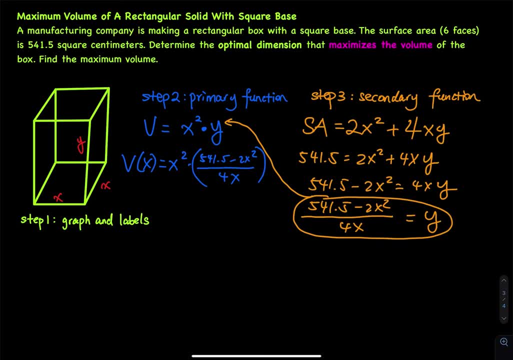 And then how do I want to rewrite this? I will just distribute the x squared. so once you distribute the x squared, you have v of x, that is equals to 541.5 divided by 4,, that is equals to 135.375,. I know the number looks weird, but when you keep moving, 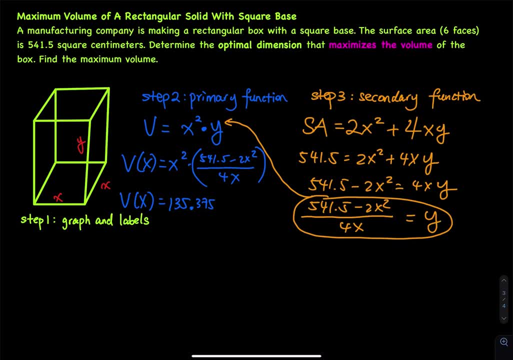 you will see that y, I pick 541.5, and then you have x squared divided by x. so you only have 541.5 divided by 4x. one x left and then minus uh, and then you distribute the x squared to the two x squared. so 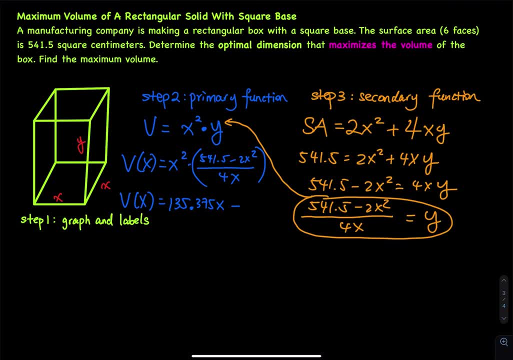 you have a two x to the fourth divided by four x, so you have a one half, and then x to the fourth divided by x, that is, x to the third. then here is your primary in terms of one independent variable. so now the primary is done and then we will move on to, we will move on the derivative. so let's move. 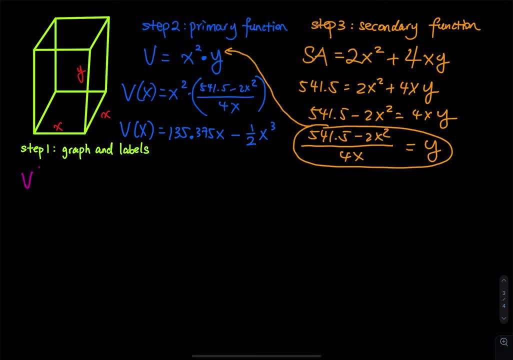 on to the derivative and then we have v, prime of x. so v, prime of x. uh, let me just call that a step four. right one, two, three and then step four is derivative and critical number and critical number and then step five. we will prove that that critical number is a min or max, right? so v. 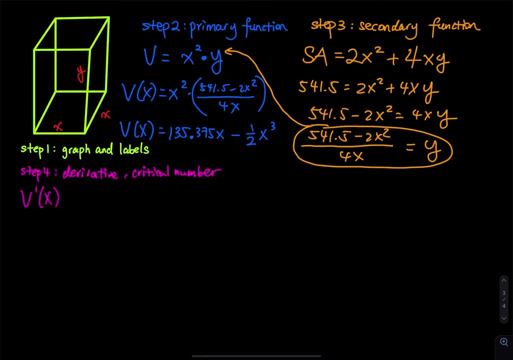 prime of x: v. prime of x that is equal to: uh, one, two, three, 35.375. the x is gone, and then you bring the three down right, so we have three over two and then x squared. what do we do next? we have to set that equals to zero. why, so? let's say: um, you have a. 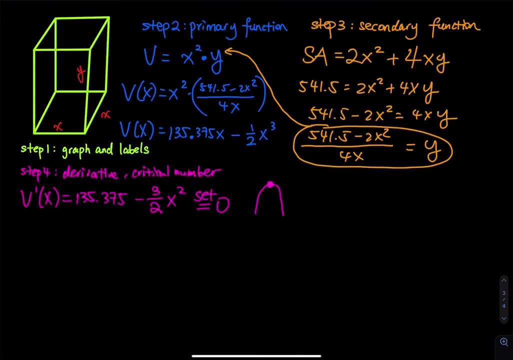 parabola. and then this is the vertex right. that is supposed to be the maximum. and then, since that is a vertex, at that point we have a horizontal tangent line. therefore the slope is equals to zero. as long as you can prove increasing and then decreasing, then that point is called maximum. so before you prove the increasing and decreasing, 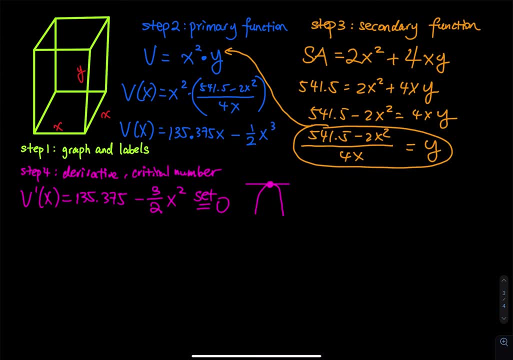 stuff. you have to show that at that point we have a horizontal tangent line and then the slope is equals to zero. so that's why you have to set the first derivative equals to zero. okay, so let's erase that. and then now we have to solve for x. uh, let's push the 135 to the right hand side, so we 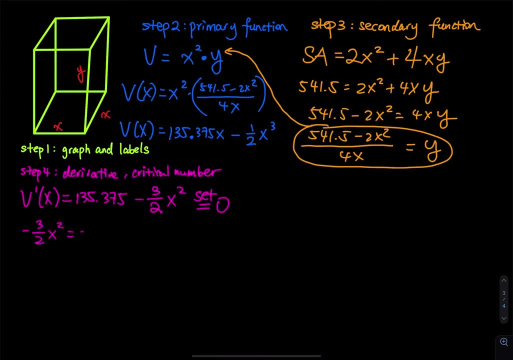 have negative. three over two x squared equals to negative 135.6, 0.375. multiply both sides by negative one, three over two x squared equals to 135.375, and then x squared is equals to 135.375. and then we times x divide, times two, divided by three. 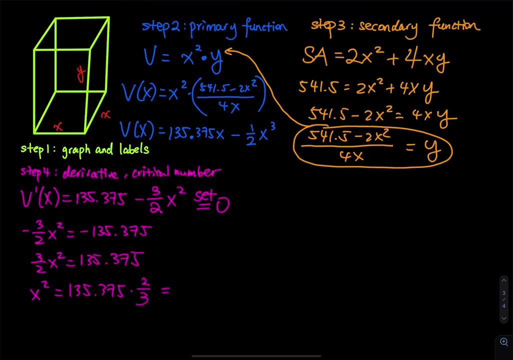 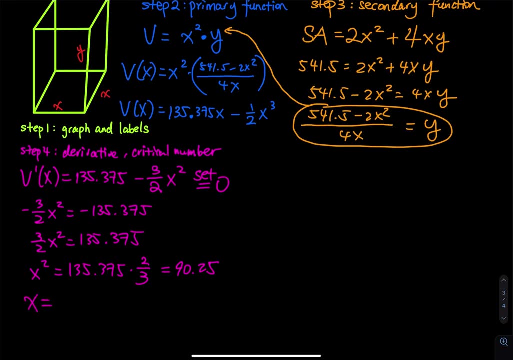 times two, divided by three, so that is equals to 90.25. so that's why i picked these numbers, because when you take the square root on both sides, the square root of 90.25, that is, equals to 9.5, exactly. so this is centimeters. so that is your x, and then this: 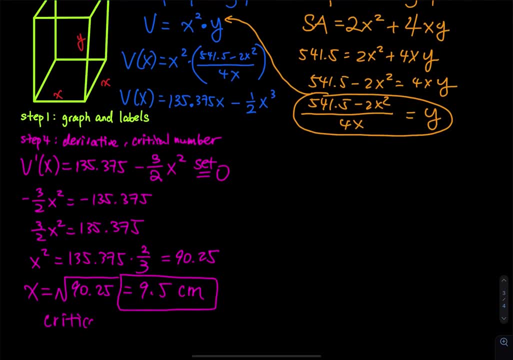 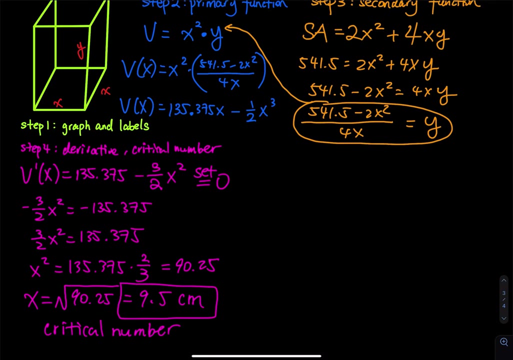 is also the critical number. i cannot call this number the absolute min or max yet, because i have to prove it okay. so, uh, now we get a critical number. how do you prove that this critical number is the absolute maximum? do you want to go by the domain or you want to go by the? 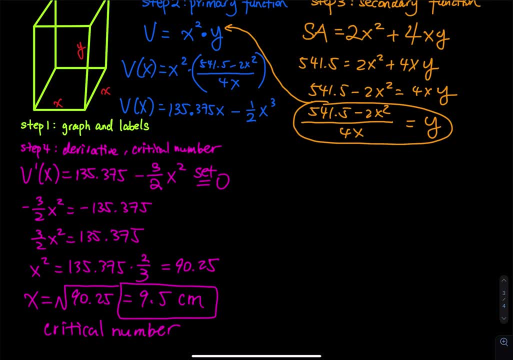 second derivative. so here is one thing that you have to know: sometimes the domain is easier, sometimes the second derivative is easier, but in some problem, when you state the domain, the domain doesn't make too much sense. so let me show, show you what. what do i mean by that? so let's move on. 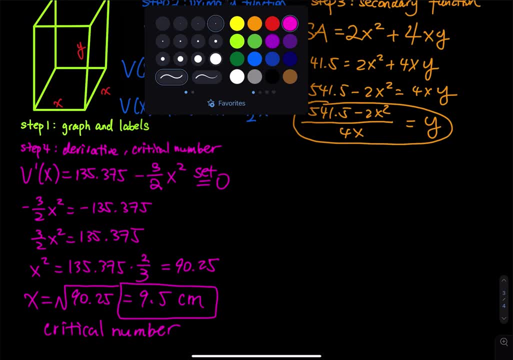 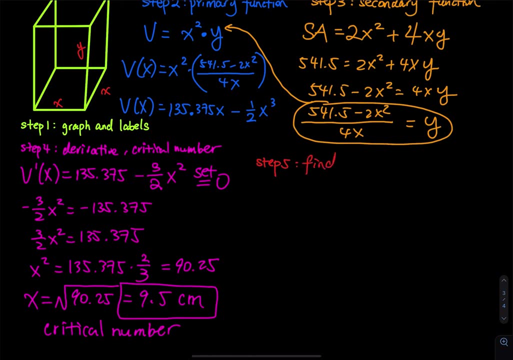 to the next step. uh, next step, let's use a red. so the next step is step five. so you have to find the min or max, right? so if you use domain, uh, the smallest x is of course zero. right, it's the smallest domain. of course that is a zero. what is the biggest value of x? how large can x be? so in this problem, 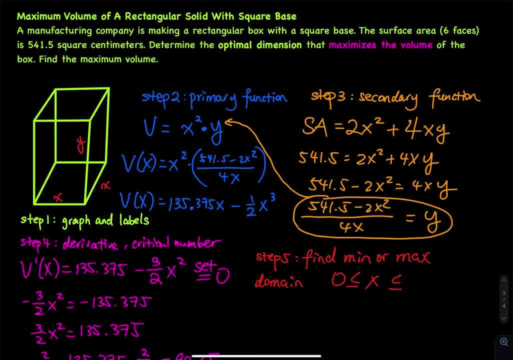 we only have one number, that is 541.5, and that is a surface area. so this is a surface area using this number. so if you want to determine the x, you can only do this 541.5. but i am not going to go go this way because that doesn't make too much sense. so when x is 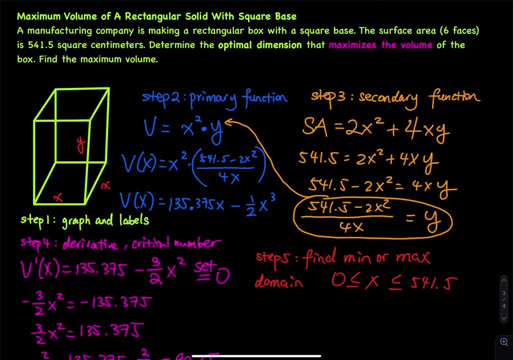 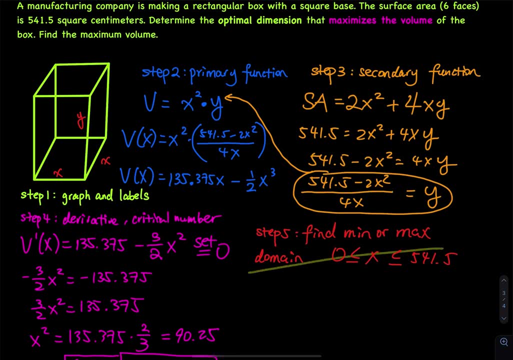 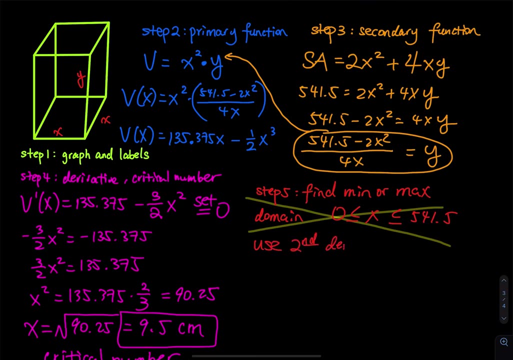 equals to 541.5. what does that mean? that doesn't make make sense to me, so that's why i am not going to use the domain. so in this problem, i am not going to use the domain. let's use the second derivative. so let's use second derivative test. to me, second derivative test is way easier because when 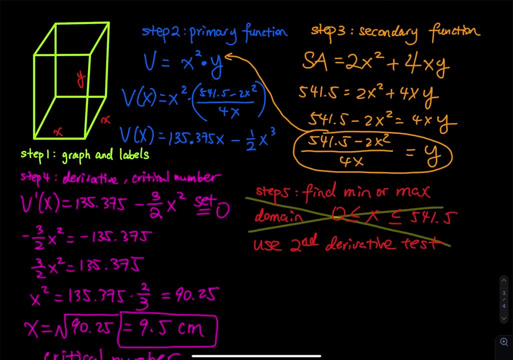 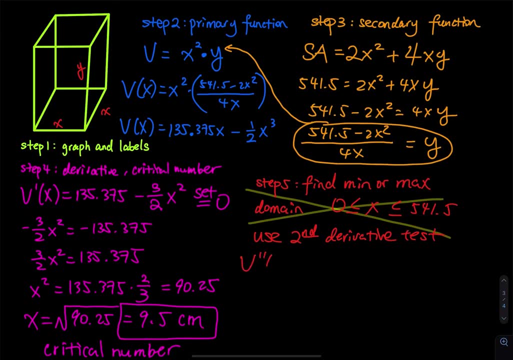 you solve this kind of optimization problem. the function is so simple you can easily get the second derivative, so we have the first prime right over here. so what is double prime, double prime? so the 135 will be gone, and then you take the na, you take the two down, so you have a negative three. 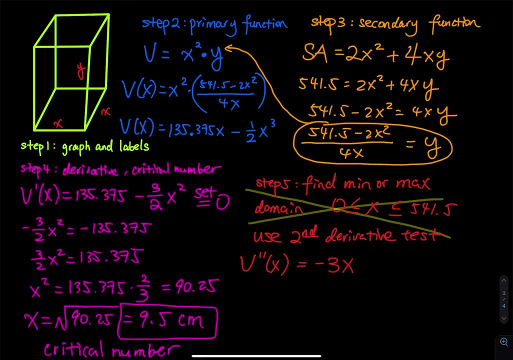 right. and then x two minus one is equals to one. that's it. look how simple it is. and then when x is equals to nine nine point five, so double prime x is equals to nine point five, we have negative three times nine point five. i don't. 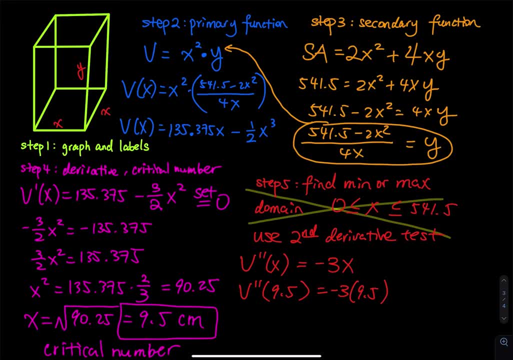 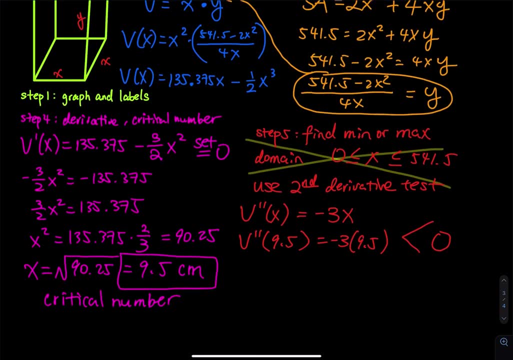 really care what that equals to, because all i need to know is that is less than zero. second derivative less than zero. what is that means? second derivative less than zero? that means the volume function. so function v is concave down. at x equals to 9.5. give me a picture. so this is a concave down. and then when x is equals to 9.5, 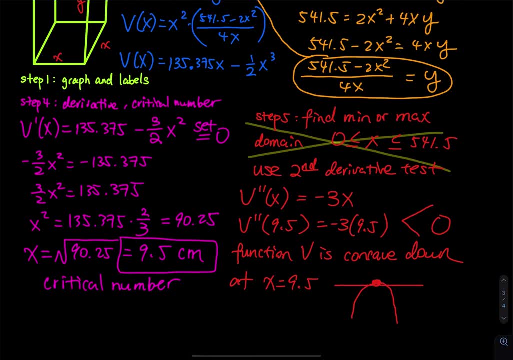 look at the first derivative. we have a horizontal tangent line right horizontal tangent line concave down. is the uh, is the critical number a max or min, clearly. so this is an absolute max. right at x equals to 9.5. that's how easy the second derivative test is. so now we just figure out that. 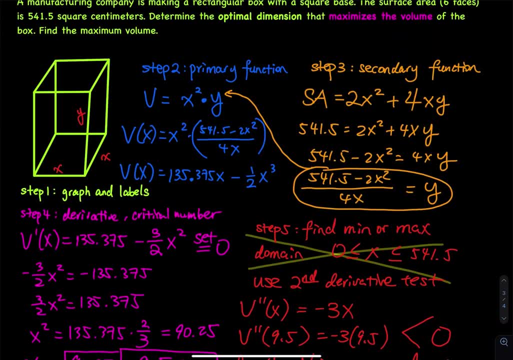 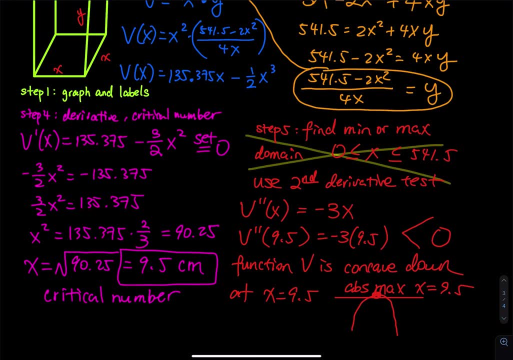 the volume. right right, the volume is maximized when x is equals to 9.5. okay, then, what is y equals to do? you see that we have a y over here. so you see that we have a y over here. so we have a y over here. so we have a y over here, so. 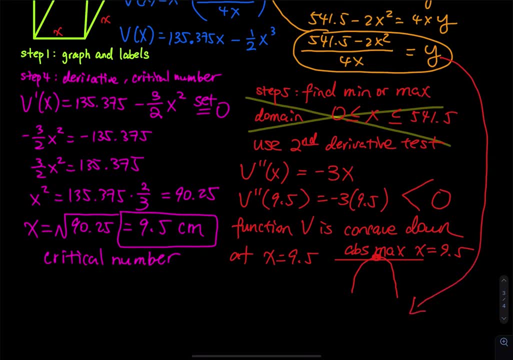 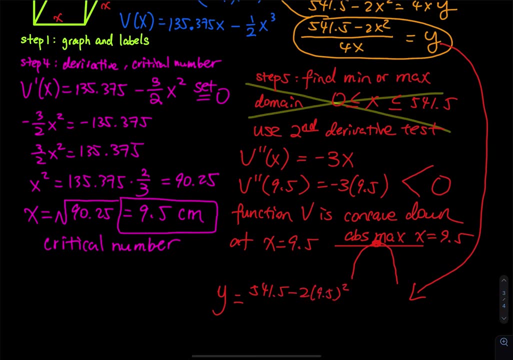 let's bring bring this down. so when x is equals to 9.5, so y is equals to 541.5 minus 2 times 9.5. square divided by 4 times 9.5, or one thing that i have to remind you is this: one works perfectly. 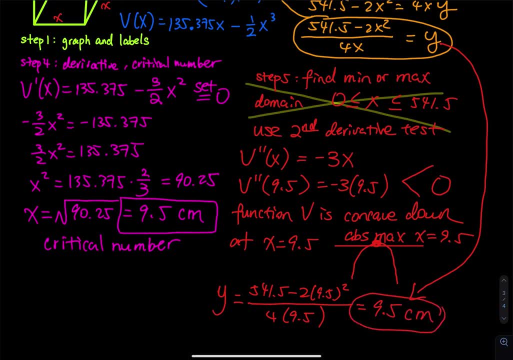 fine, so it's just 9.5 centimeters. but sometimes you will get a very weird function that will, when you take the top divided by the bottom, you will just get an approximation. so listen to me right now, do when, especially when you are doing homeworks and exams online. so, especially when you're doing 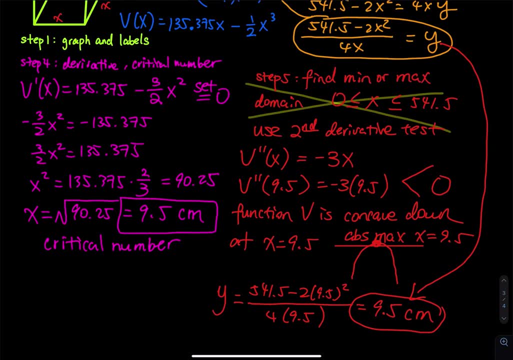 works online. do not submit the approximation unless the question let you do so. okay, once again, do not input the approximation and click submit unless the problem allows you to do so, because most of the time they will just take an exact value. they don't take approximation. when you report this to your boss, you can report the approximation and you will get an exact value. 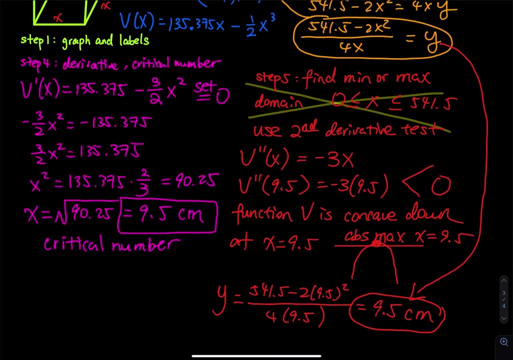 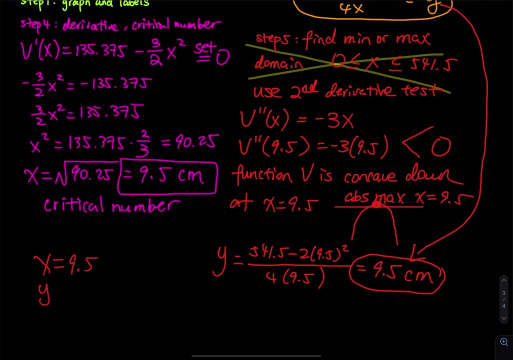 but when you are reporting these answers to an online homework or exam system, they only accept exact answer to approximation. even though you get it right, they will just mark it wrong. okay, so be very careful. so this one, x is equals to 9.5, y is equals to 9.5 and 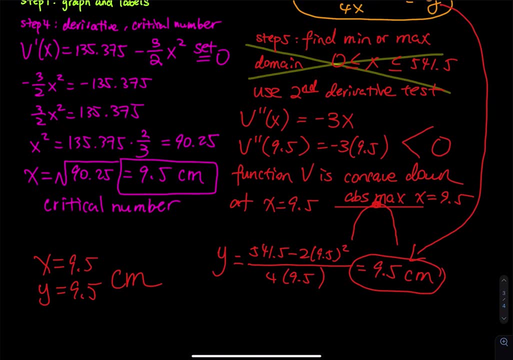 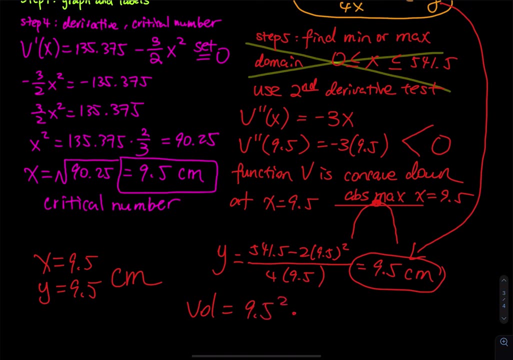 they are both centimeters. and then what about the volume? so the volume is equals to the base right. the base is 9.5 square and then you multiply 9.5, that is equals to 857.375. the volume is in cubic centimeters, so cm3, so cubic centimeters. 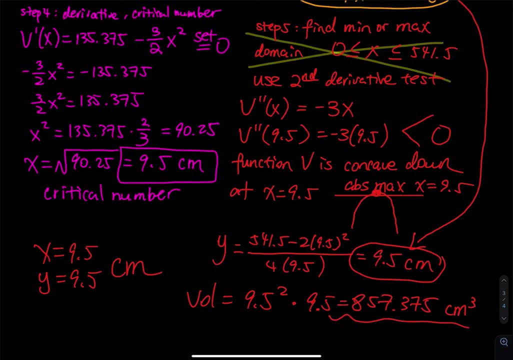 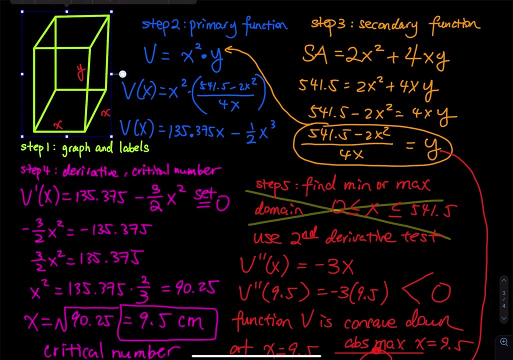 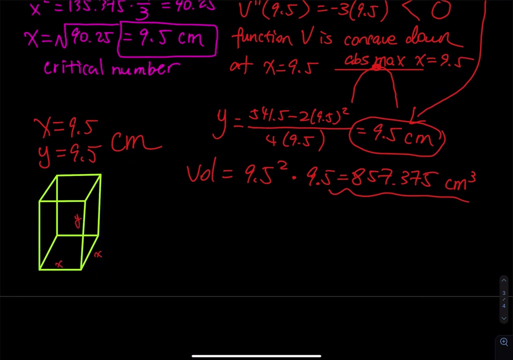 so when you report this, you have to report x equals to this, y equals to that, and then report the volume to your boss. and then i will just do one more work to impress my supervisor by doing this. i will just put copy and paste and then put this picture right next to it. so you are trying to 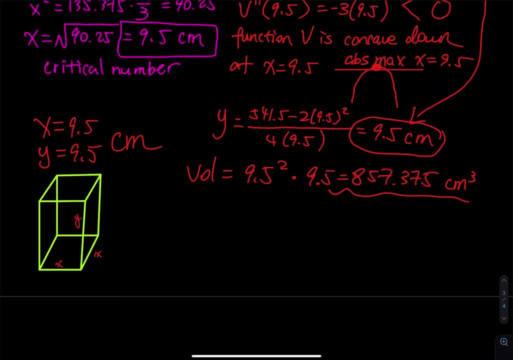 do this, x and y both equals to 9.5, and then here is your maximum volume. i will just provide this to my supervisor. okay, so that is the end of this problem, do you like it? is this helpful? if so, give me a like, share and subscribe, and i will catch you all in the next lesson signing out.